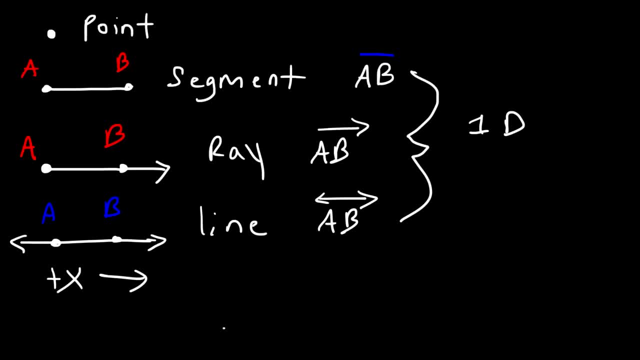 travel in the x-direction for a horizontal line. Now, a plane is two-dimensional. You could travel in the x-direction or you could travel in the y-direction. So a plane is flat as a pancake And like a line, it extends infinitely into the x and y-directions. Now what is the difference? 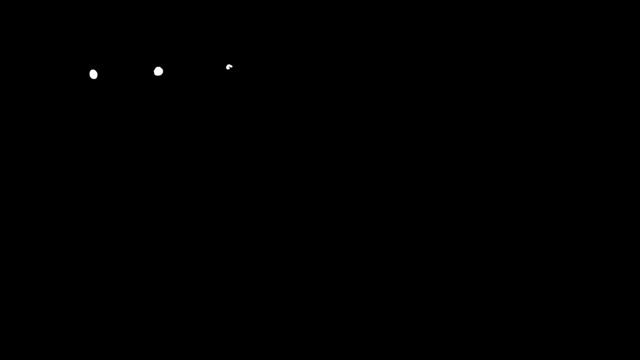 between collinear points and non-collinear points. So let's call this point A, B and C. Three points are collinear if they lie on the same line, So these are known as collinear points. Now the other three these points are: 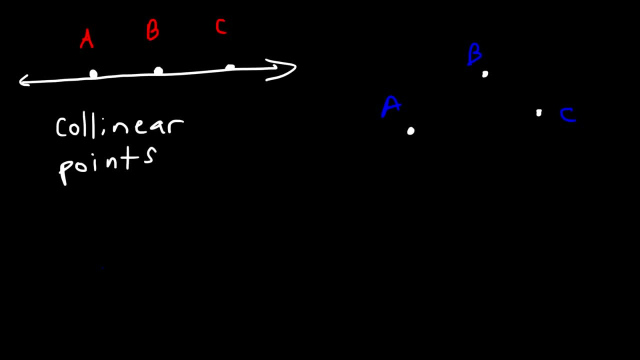 points are non-collinear because we cannot draw one line that connects all of them. we can draw a line between two points so we can say AB is collinear, but A, B and C are not collinear because we can't put those three points in a single. 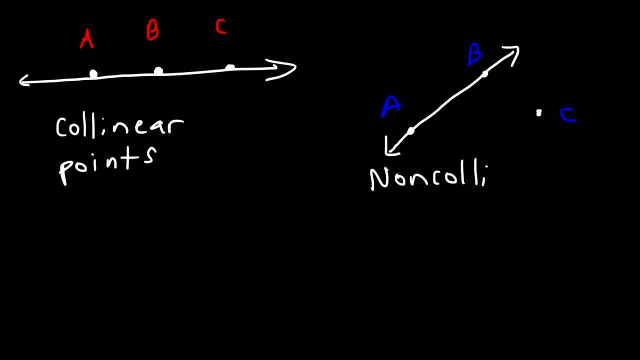 line, so these are known as non-collinear points. now let's say, if we have four points that lie on the same plane, let's call this point A, B, C and D. These four points are known as coplanar points because they share the same plane, and let's call this plane X. 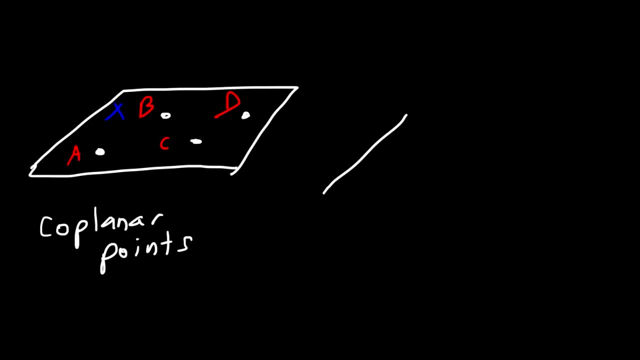 and let's call this plane X, and let's call this plane X. let's say this is A, B, C, D. So these four points are known as non-coplanar points because they do not lie on the same plane. A, B and C lie on the plane. 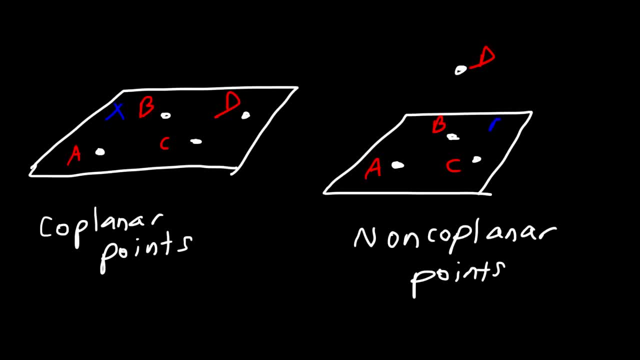 but D is outside of the plane. so if we call this plane M, we can say A, B and C are located on plane M, but D is not on plane M. so those are known as non-coplanar points. Now there are four ways to determine the existence of a plane. the first method is three. 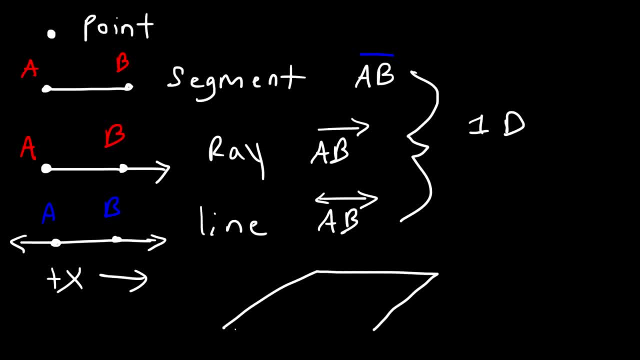 Now a plane is two-dimensional. You could travel in the X direction or you could travel in the Y direction. So a plane is flat as a pancake and like a line it extends infinitely into the X and Y directions. 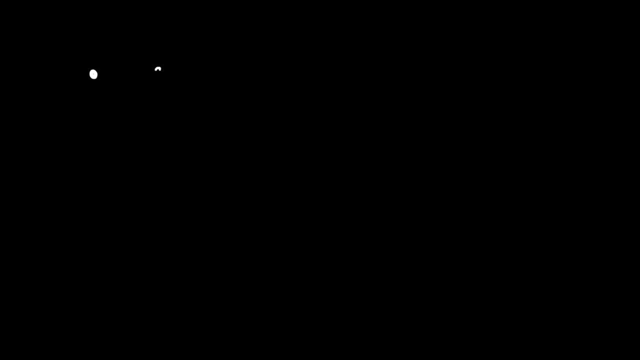 Now, what is the difference between collinear points and non-collinear points? So let's call this point A, B and C, 3D, 3D, 3D points are collinear if they lie on the same line, So these are known as collinear points. 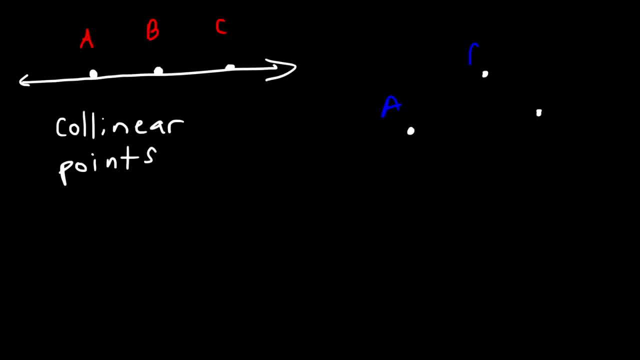 Now the other three. these points are non-collinear because we cannot draw one line that connects all of them. We can draw a line between two points so we can say A, B is collinear, but A, B and C are not collinear because we can't put those three points in a single line. 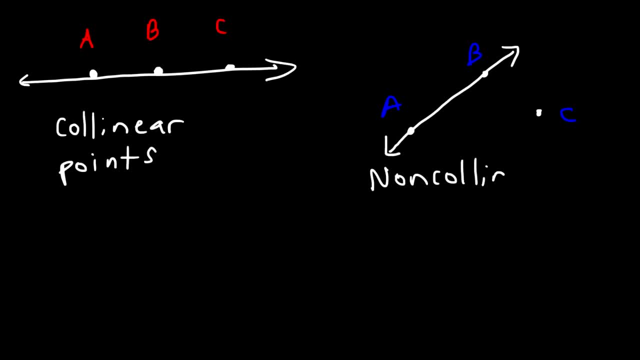 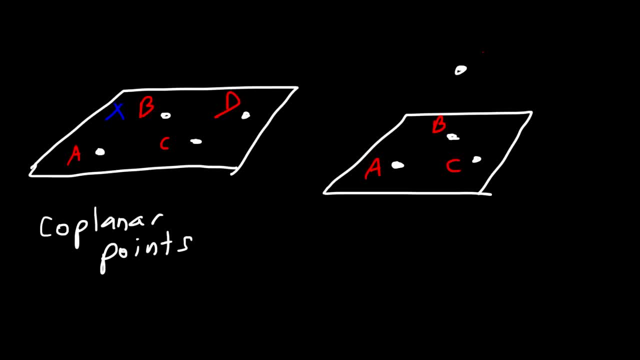 Let's say this is A, B, C, D. So these four points are known as non-coplanar points because they do not lie on the same plane. A, B and C lie on the plane, but D is outside of the plane. 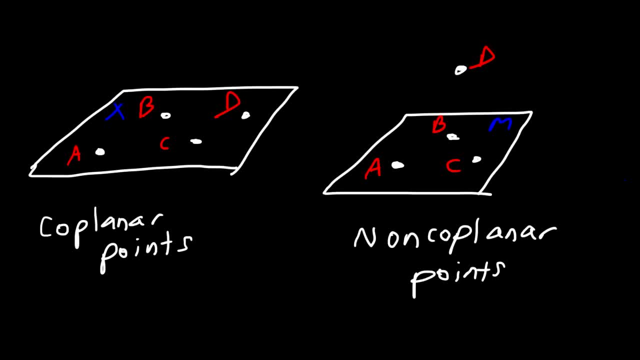 So if we call this plane M, So if we call this plane M, we can say A, B and C are located on plane M, but D is not on plane M. So those are non-coplanar points. 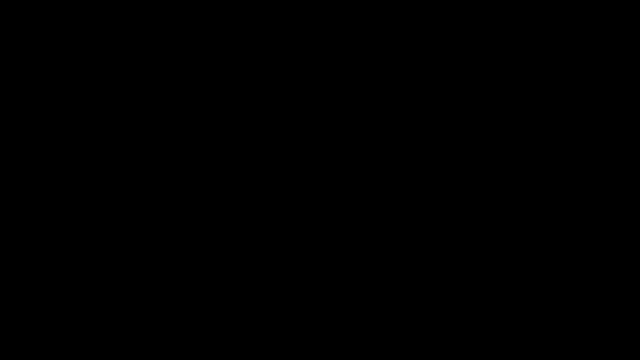 Now there's four ways to determine the existence of a plane. The first method is three non-collinear points. There's always exactly one plane that can pass through three non-collinear points. So that's the first method. The second method is a line N of 1.. 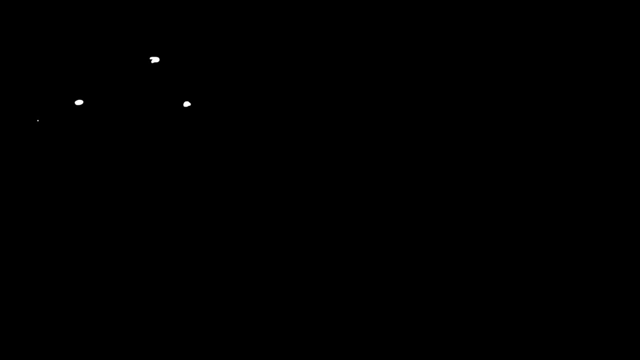 non-collinear points. There's always exactly one plane that can pass through three non-collinear points, so that's the first method. The second method is a line and a point. only one plane can pass through a line and a point point, So let's call this line M and point A. The third method is two parallel. 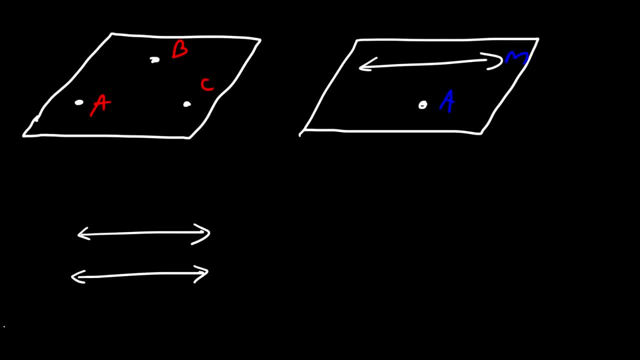 lines. Let's call this line L and line K. Only one plane can pass through two parallel lines, and so these two lines are known as coplanar lines, because they lie on the same plane. Now, two lines that intersect also lie on one plane, so 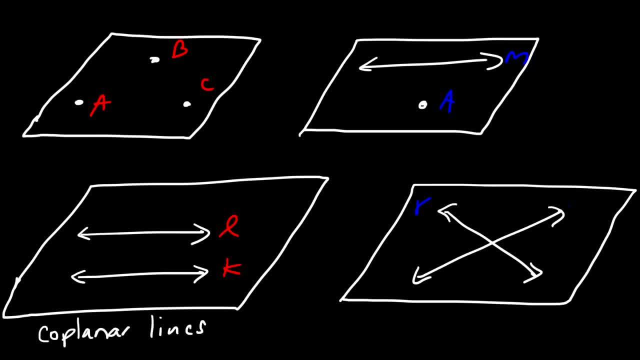 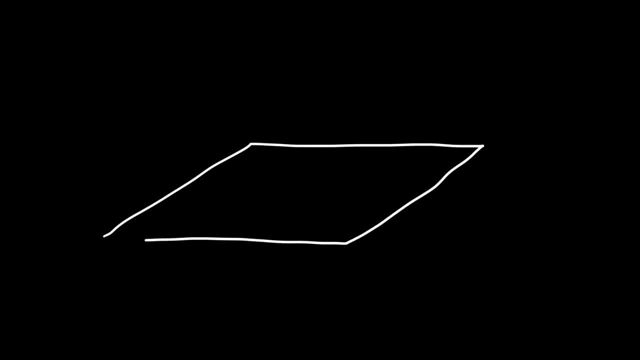 let's call this line R and line S. They intersect at this point and so these two are coplanar lines. They share the same plane. Now you can also have non-coplanar lines. For example, let's say this is line L and let's say: if we have a line perpendicular, 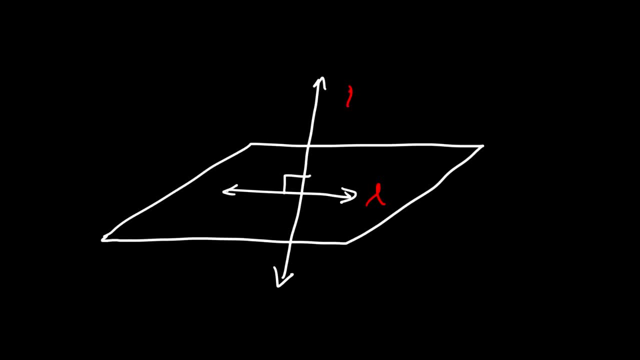 to it. let's call this line K. So line L lies on plane M, but line K does not, So these are known as non-coplanar lines. Now let's say, if we have plane Y and then we have these points. 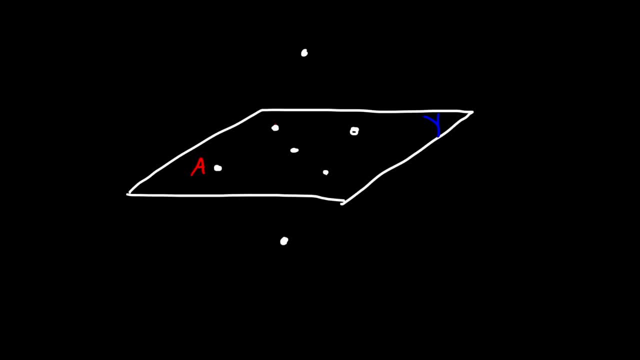 Let's call it points A- Actually I'm going to make this A, B, C, D. Let's say this is E, F and G. So which of these points are coplanar points? The coplanar points are the points lying on plane Y. 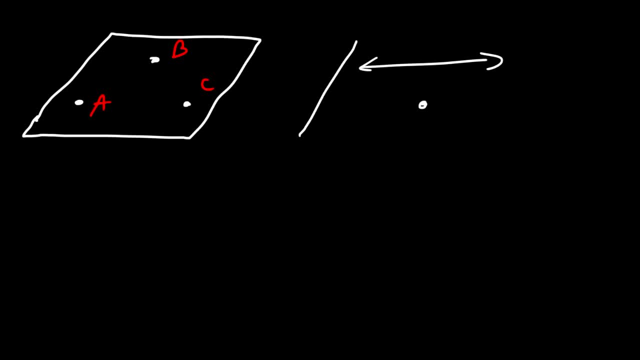 And a point. Only one plane can pass through a line and a point, So let's call this line M and point A. The third method is two parallel lines. Let's call this line L and line K. Only one plane can pass through two parallel lines. 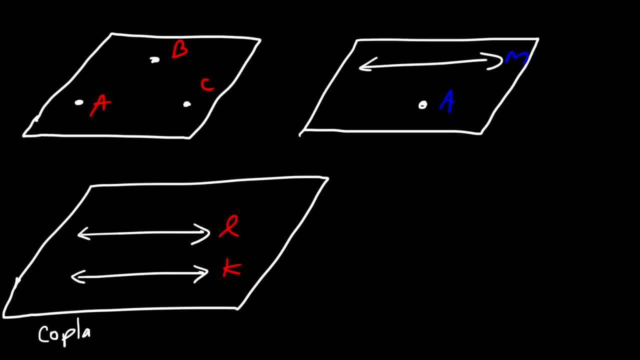 And so these two lines are known as coplanar lines, Because they lie on the same plane. Now, two lines that intersect also lie on one plane, So let's call this line R and line S. They intersect at this point. 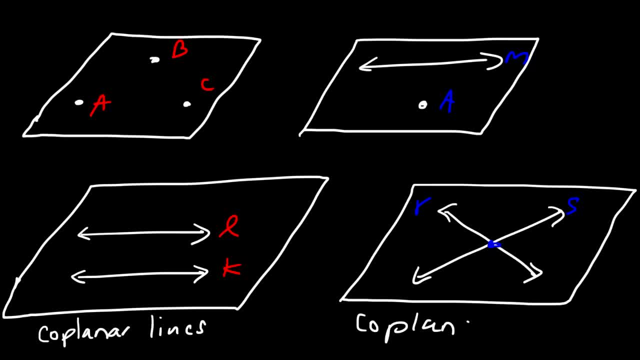 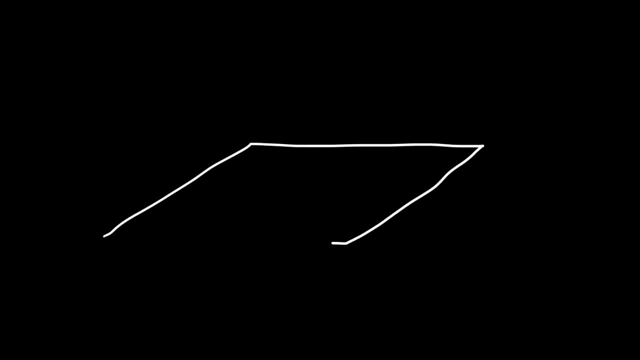 And so these two are coplanar lines. They share the same plane. Now you can see that these two lines are non-coplanar. Now you can also have non-coplanar lines. For example, let's say this is line L. 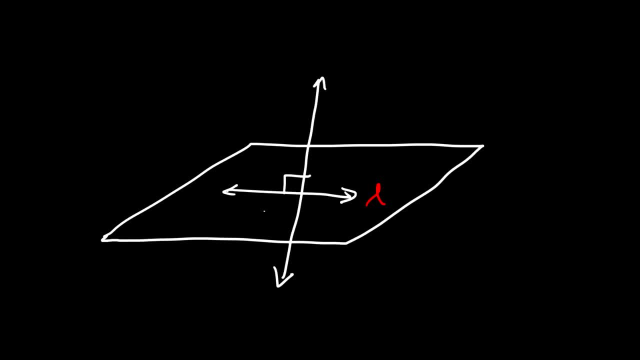 And let's say: if we have a line perpendicular to it, let's call this line K. So line L lies on plane M, but line K does not. So these are known as non-coplanar lines. Now let's say: if we have 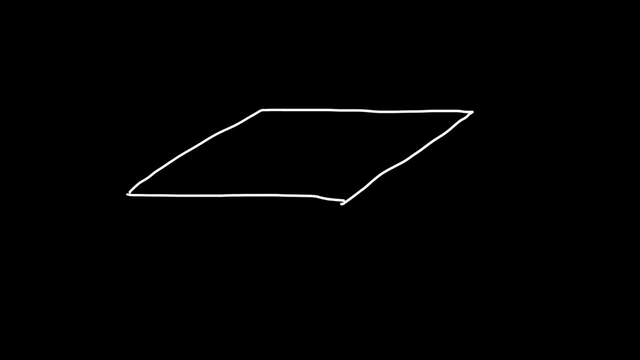 Plane Y. And then we have these points. Let's call it points A, A- Actually, I'm going to make this- A, B, C, D. Let's say this is E, F And G. So which of these points are coplanar points? 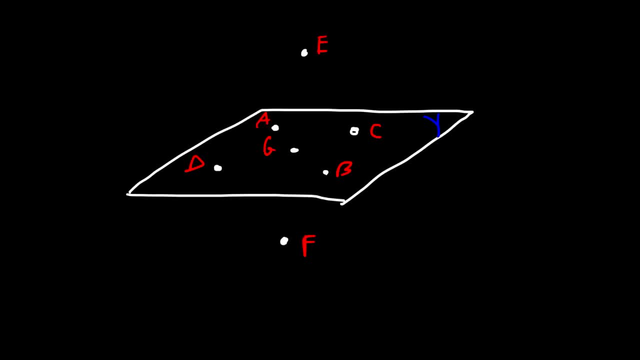 The coplanar points are the points lying on plane Y. So A, B, C, D and G are coplanar points. These five, The non-coplanar points, would be these five along with E, Or along with F. 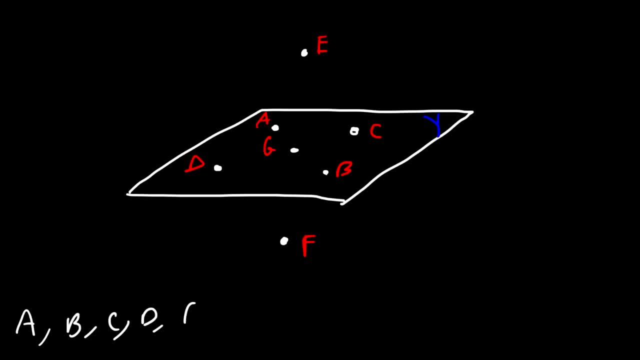 So A, B, C, D and G are coplanar points. these five, The non-coplanar points, would be these five along with E or along with F. So combined these seven are non-coplanar points. These five are coplanar. but once you add E to the mix or F to the mix, 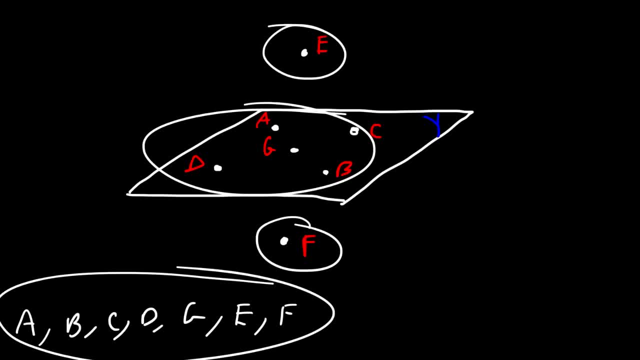 then they're considered non-coplanar points because these points are not all on the same plane. So make sure you understand that. So these five are coplanar points. These six are non-coplanar points because E is not on plane Y. 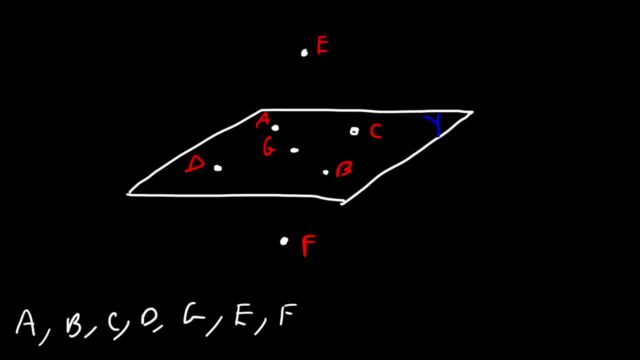 And these seven points are also non-coplanar points. Now identify the coplanar lines in this example. So we could say that line CD and line AB are coplanar lines because they exist on the same plane. Okay, Now if we add top microplanes? 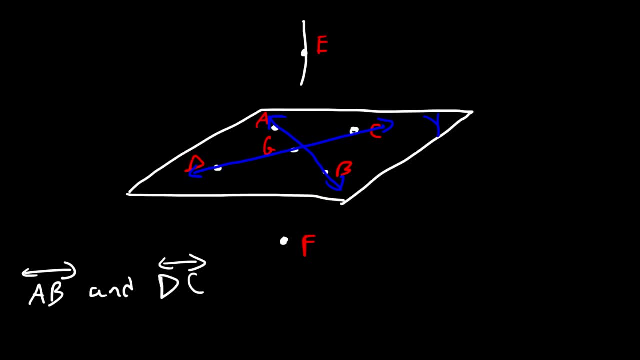 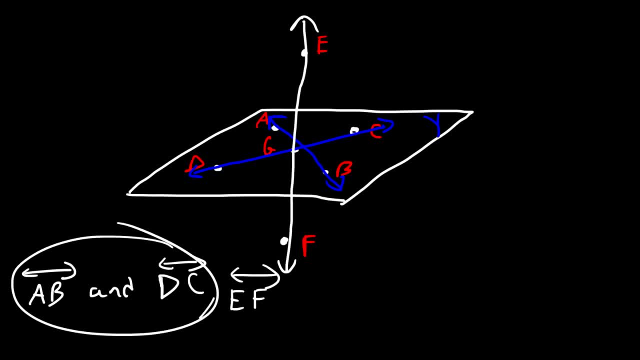 AB and DC are coplanar lines. they exist on plane Y, but all three of these, once you add EF to the mix, then it's considered to be non-coplanar lines. they don't share the same plane. Now. 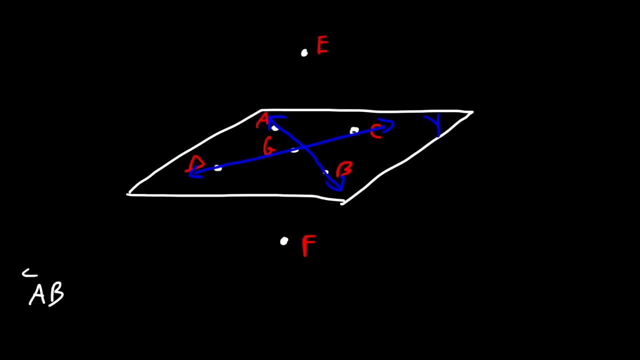 what about coplanar segments? Well, the answer would be the same as coplanar lines. So segment AB, which starts here and ends here, is coplanar with segment DC. However, segment EF is non-coplanar with AB and DC. So you can have coplanar segments and non-coplanar segments. So I'm going to give 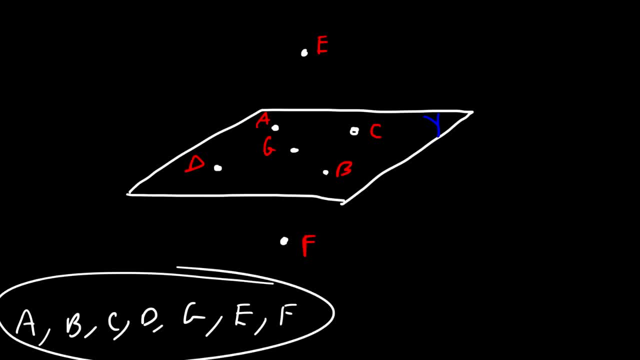 So, combined, these seven are non-coplanar points. These five are coplanar but once you add E to the mix or F to the mix, then they're considered non-coplanar points, because these points are not all on the same plane. 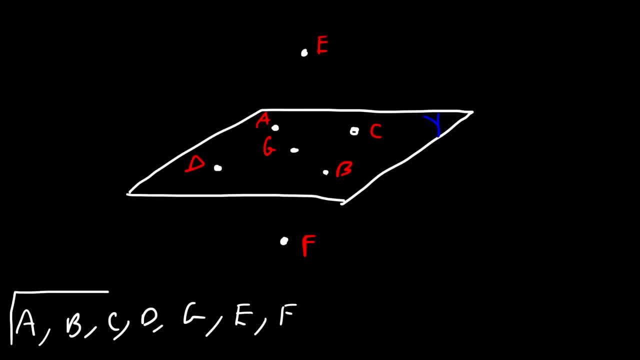 So make sure you understand that. So these five are coplanar points, These six are non-coplanar points because E is not on plane Y And these seven points are also So non-coplanar points. Now identify the coplanar lines in this example. 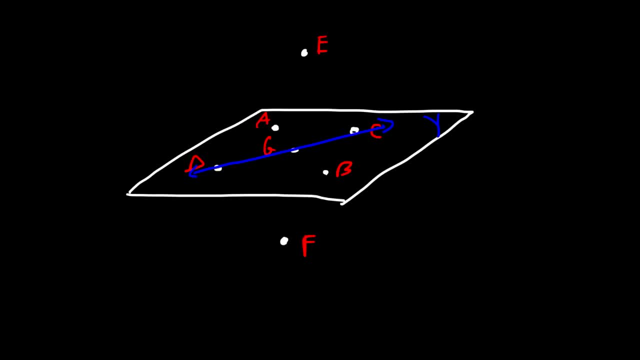 So we could say that line C, D and line A, B are coplanar lines Because they exist on the same plane. Now if we add- let me draw that better, let's say line E, F to the mix, 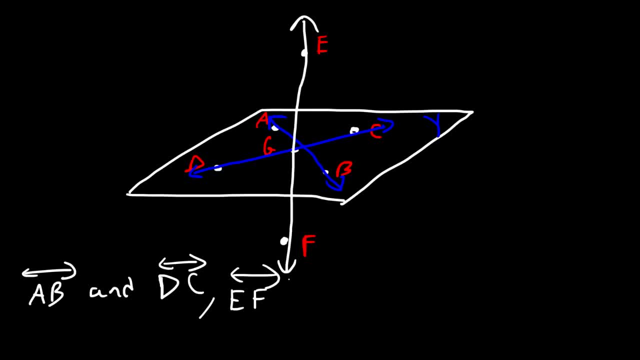 Then these three are non-coplanar lines. A, B and D C are coplanar lines. They exist on plane Y, But all three of these, once you add E, F to the mix, then it's considered to be non-coplanar lines. 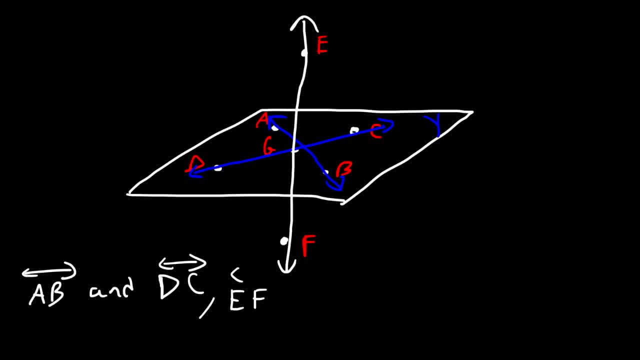 They don't share the same plane. Now, what about coplanar segments? What about coplanar segments? Well, the answer would be the same as coplanar lines. So segment A, B, which starts here and ends here, is coplanar with segment D, C. 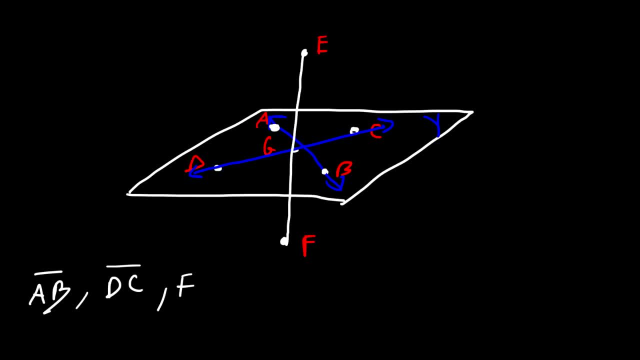 However, segment E F is non-coplanar with A, B and D C, So you can have coplanar segments and non-coplanar segments. So I'm going to give you some verbal questions regarding these two planes. 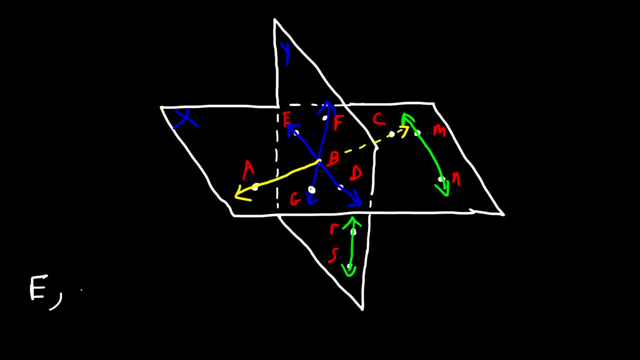 So I'm going to give you three points. Points E, D and C determine which of the two planes, plane X or plane Y. Now notice that point D, E and C, they're all located within plane X. 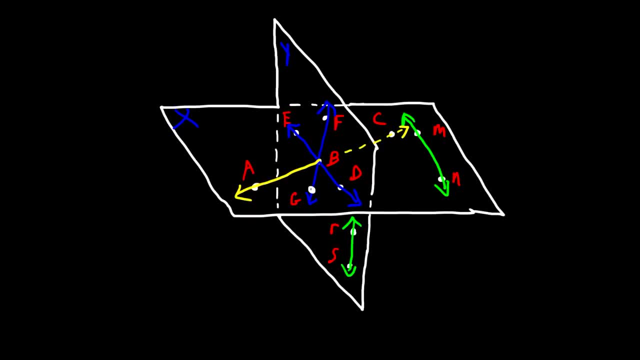 you some verbal questions regarding this. So I'm going to give you three points. Points E, D and C determine which of the two planes, plane X or plane Y. Now notice that point D, E and C, they're all located within plane X. So these 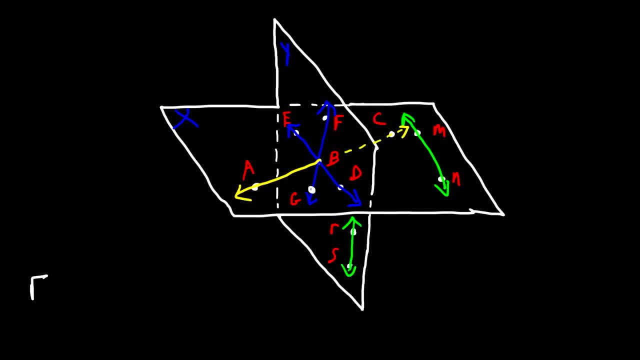 three points determine plane X. Now what about, let's say, points F, D and R? These three non-colonial points determine which plane. So F is on plane Y, not X, D is on plane X and Y And R is on Y, but not. 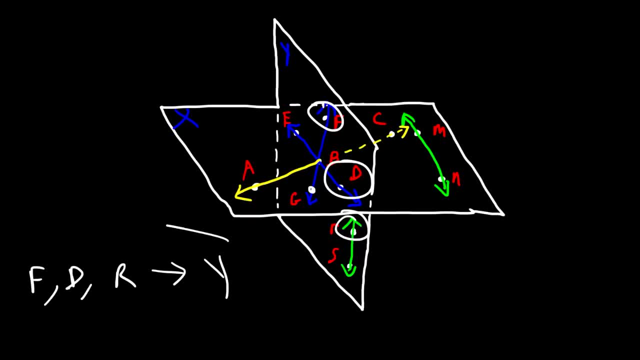 X. So these three points determine plane Y. On two lines, X and Y would get integral. So, as we could see, it takes at least three non-colonial points to determine a plane. Now we can also determine a plane using two lines. So line ED and line AC determine which. 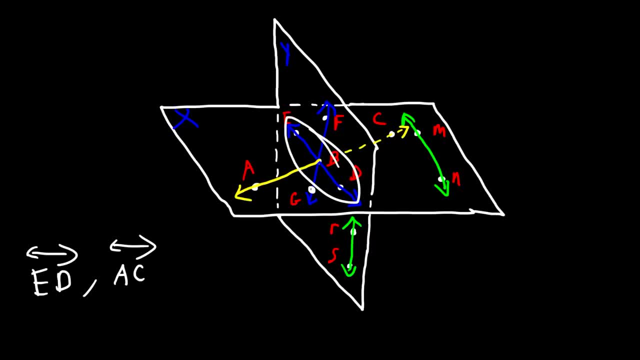 plane. So ED is in both planes X and Y. wonder why in plane X and not plane Y. So these two lines are found in plane X, So X is the answer for this example. Now, what about line ED and line FG, These two lines? 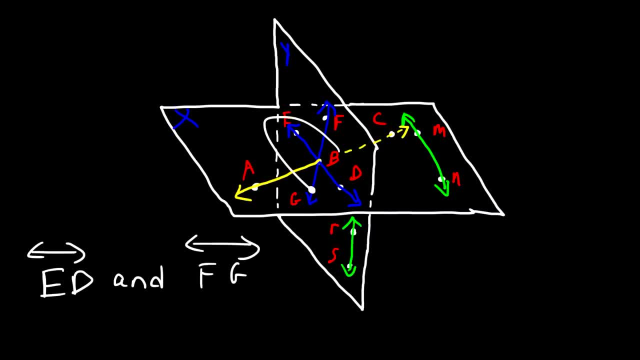 determine which plane? So, as we said before, ED is found in both planes, but FG is found in plane Y and not X. So these two lines determine plane Y. Now here's a question for you. Point A lies: on which plane Determine the planes that each of? 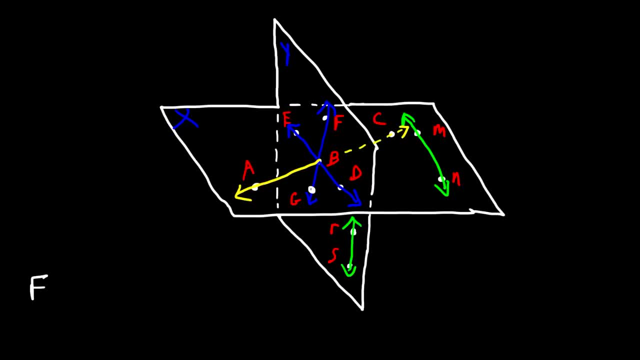 So these three points determine plane X. Now what about, let's say, points F, D and R? These three non-colonial points determine which plane. So F is on plane Y, not X. D is on plane X and Y. 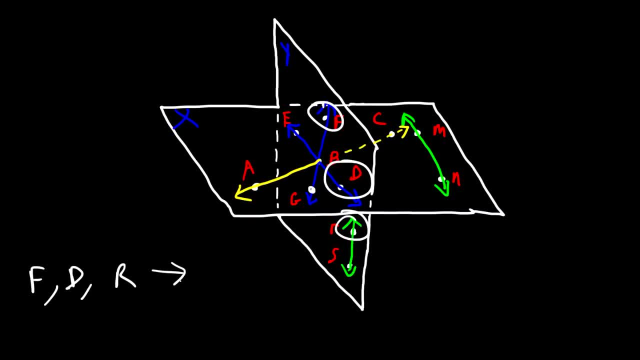 And R is on Y but not X. So these three points determine plane Y. So, as we can see, it takes at least three non-colonial points to determine a plane. Now we can also determine a plane using two lines. 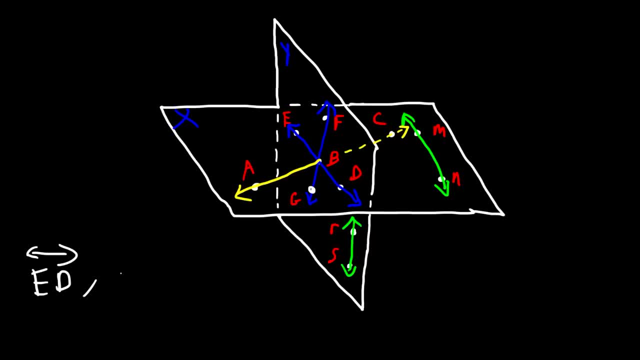 So line E D and line A C determine which plane. So E D is in both planes X and Y, But A C is in plane X And A C is in plane X and not plane Y. 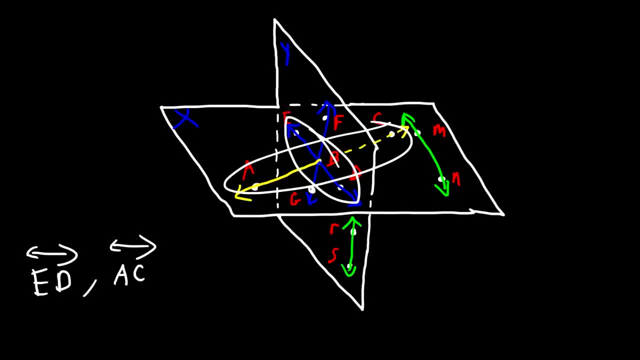 So these two lines are found in plane X. So X is the answer for this example. Now what about line E D and line F G? These two lines determine which plane. So, as we said before, E D is found in both planes. 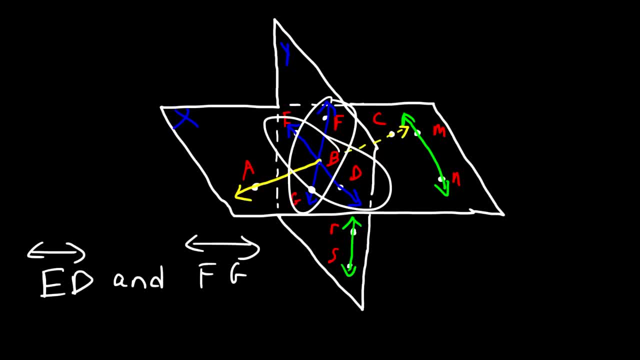 But F, G, E, D is found in plane Y and not X, So these two lines determine plane Y. Now here's a question for you. Point A lies on which plane Determine the planes that each of these points lie on? 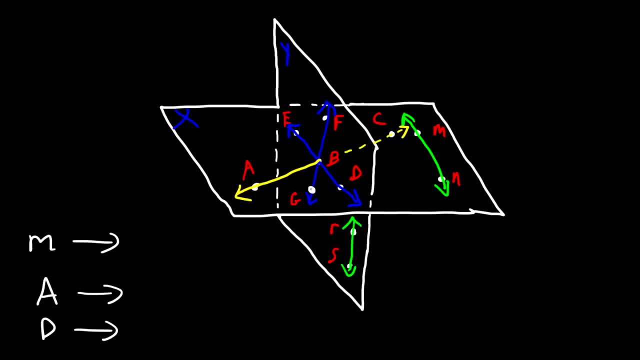 A, D, M, F and so forth, and R. So R is found in plane Y, F is also in plane Y, M is found in plane X, A is in X And D is at the intersection of X and Y. 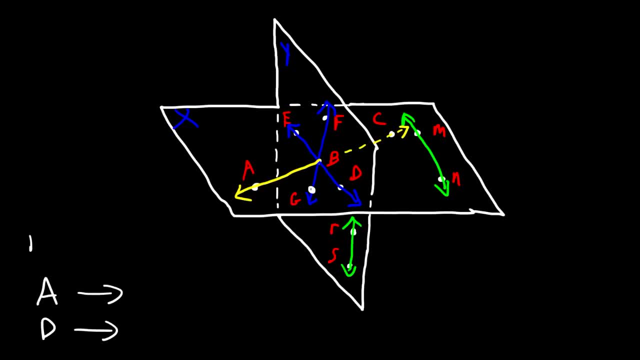 these points lie on A, D, M, F and so forth, and R. So R is found in plane Y, F is also in plane Y, M is found in plane X, A is in X And D is at the intersection of X and Y. So we can write. 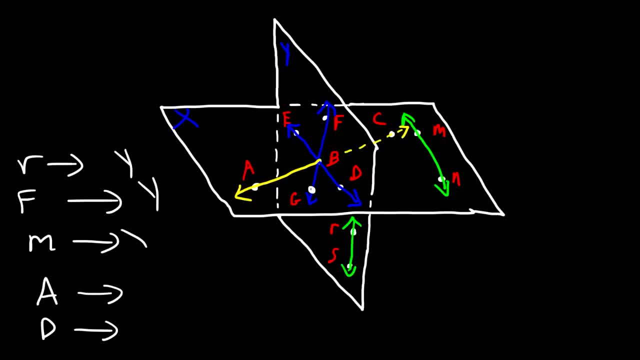 X and Y for D. Now what is the intersection of X and Y? So the intersection between plane X and plane Y is a line, And notice that line ED is found at the intersection of these two planes. So the answer for this is line ED. Now line ED and plane Y are not. 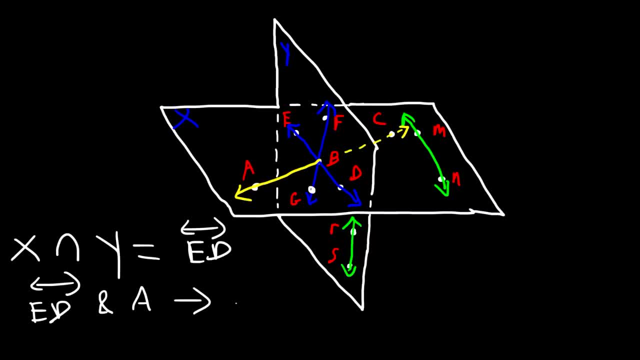 Button E D A, Point A: 15 Points N. Plane 12, Plane X 11. Plane 18. Plane X 10: 1 0, 1, 6, 3, 4, 2, 3, 2, 4. 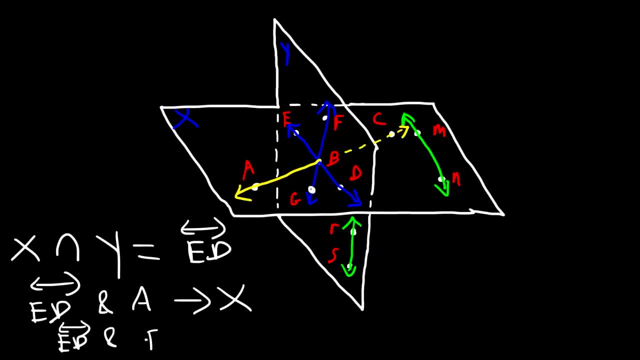 3, 1, 5, 6, 9, 2, 6, 5, 6, 5, 2, 6, 3, 6, 5, 6, 18, 10, 12, 3, 12, 2, 26, 20, 31 are coplanar with A, B, C and D. So A, B, C and D are found in plane X, So the other. 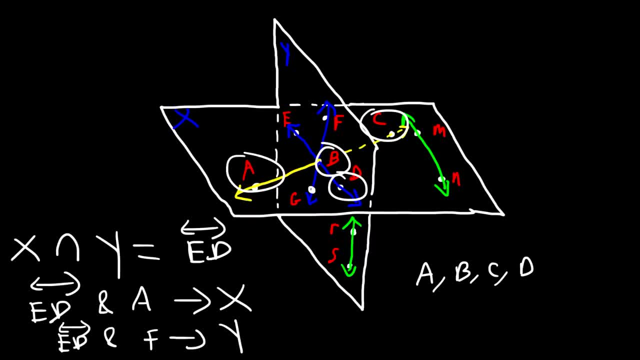 points that are coplanar with these four points are the other points that are found in plane X. So E is in plane X, G is not. M and N are in plane X. G is actually in plane Y. It's going down, So let me just mark this off. So the answer would be E, M and N. They're. 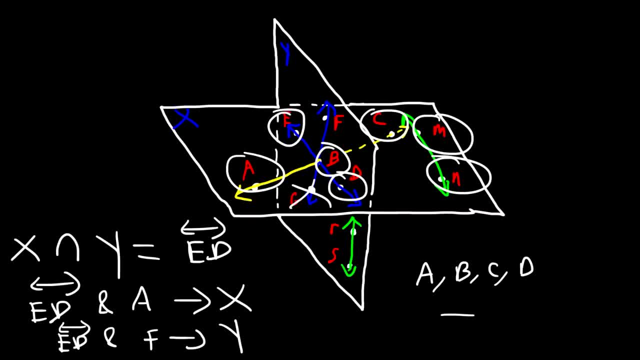 coplanar to plane X. Now, which points? oh, by the way, the other points are non-coplanar to it. So like F, G, R and S are non-coplanar to A, B, C and D. 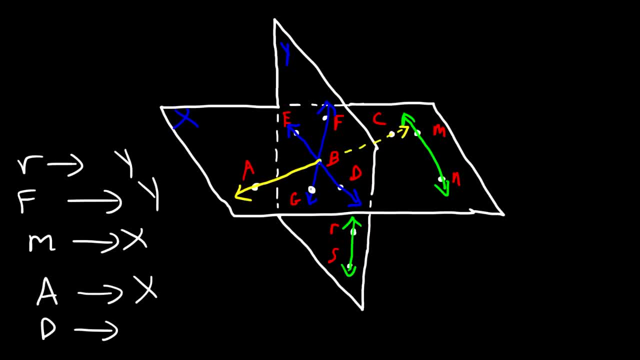 So we can write X and Y for D. Thank you. Now what is the intersection of X and Y? So the intersection between plane X and plane Y is a line, And notice that line E D is found at the intersection of these two planes. 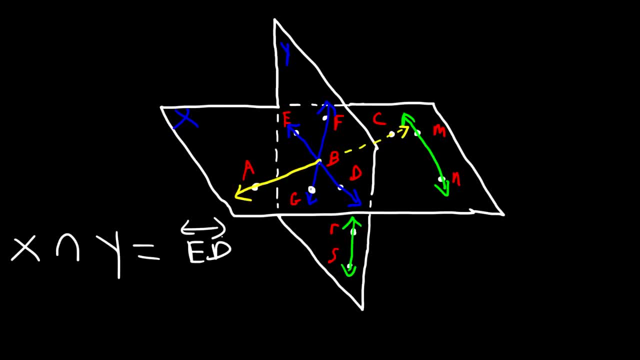 So the answer for this is line E D. Now line E D and point A determine what plane. So E D and point A are the same plane And point A. they're both found in plane X. 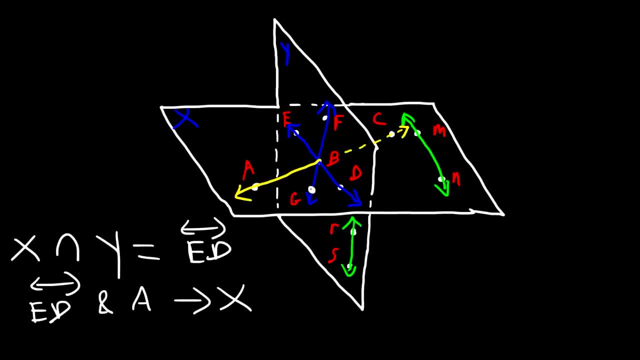 So it determines plane X. Remember, if you have a line and a point, they determine only one plane. Now, what about line E, D and, let's say, point F? F and E, D are found in plane Y. 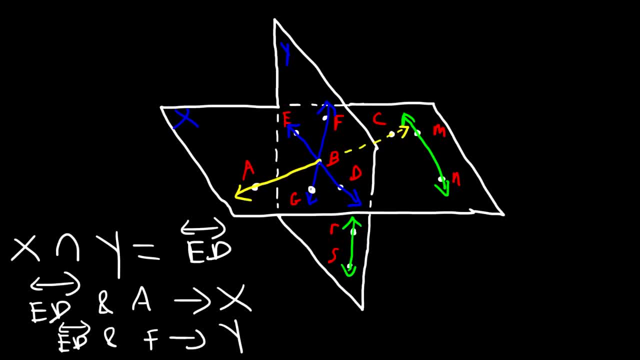 So this line and that point determines plane Y. Now, which points are coplanar with A, B, C and D? So A, B, C and D are found in plane X. So the other points that are coplanar with these four points are the other points that are found in plane X. 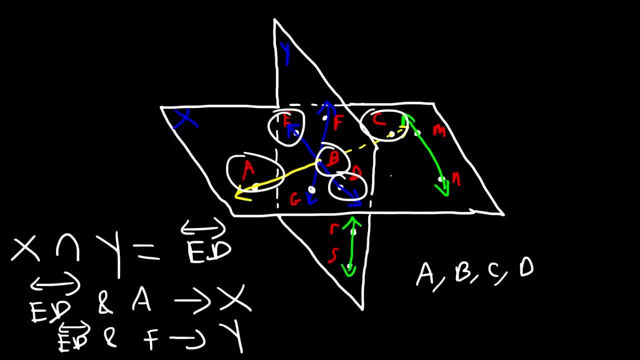 So E is in plane X, G is not. M and N are in plane X. G is actually in plane Y. It's going down, So let me just mark this off. So the answer would be E, M and N. 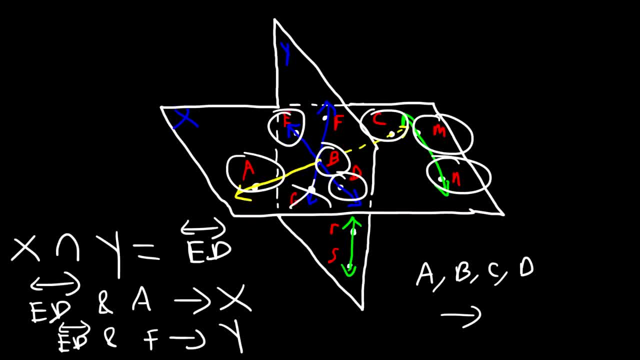 They're coplanar to plane X. Now which points? Oh, by the way, the other points are non-coplanar to it. So like F, G, R and S are non-coplanar to A, B, C and D. 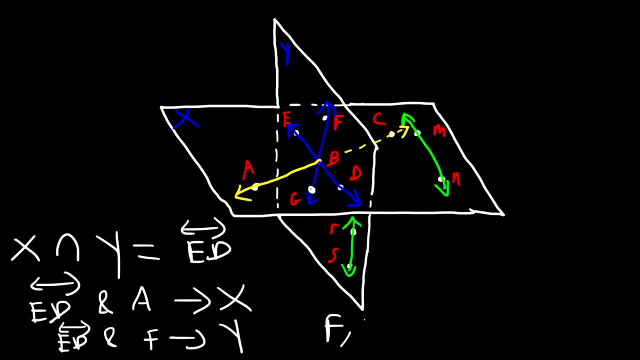 Now which points are coplanar to F, B and G? So F, B and G, they determine plane Y. So the points that are coplanar to these three points are the other points found in plane Y. 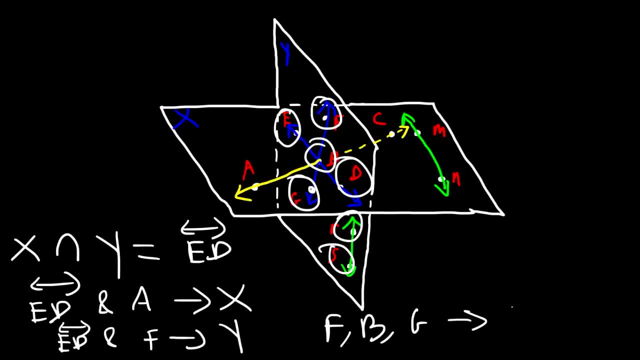 So E, D, R and S are found in plane Y. So now which points are non-coplanar to F, B and G? So which points are found in plane X but not in plane Y in plane Y? So A, C, M and N are non-coplanar to F, B and G. These three points they identify. 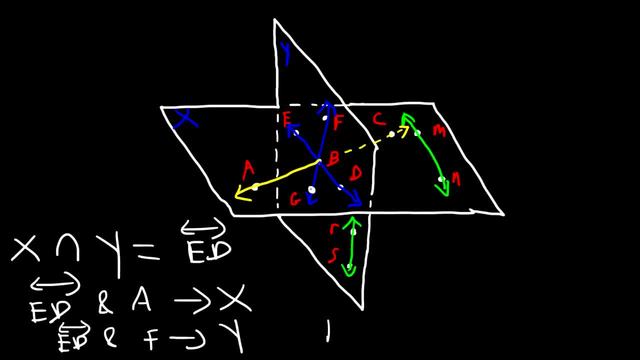 Now which points are coplanar to F, B and G. So F, B and G, they determine plane Y. So the points that are coplanar to these three points are the other points found in plane Y. So E, D, R and S are found in plane Y. So now which points are non-coplanar to A? 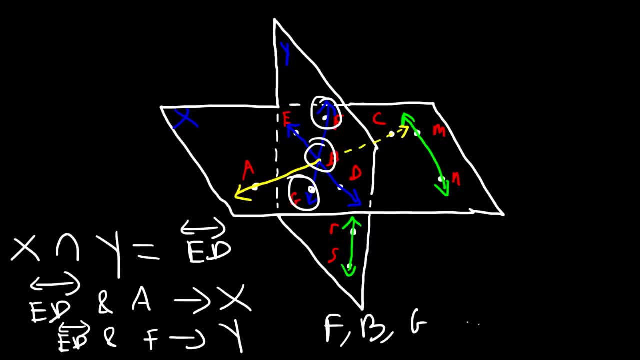 B, C and D. Now which points are coplanar to F, B and G? So F, B and G they determine F, B and G. So which points are found in plane X but not in plane Y? So A, C, M and N are non-coplanar. 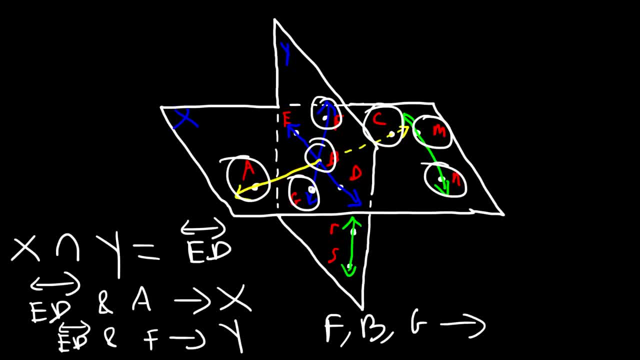 to F, B and G These three points- they identify plane Y, and A, C, M and N are not in plane Y, so therefore these points are non-coplanar to F, B and G. 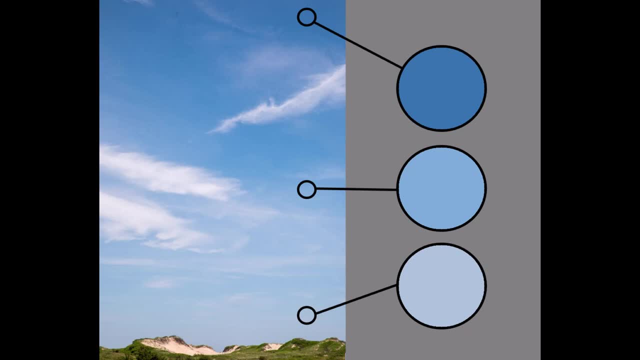 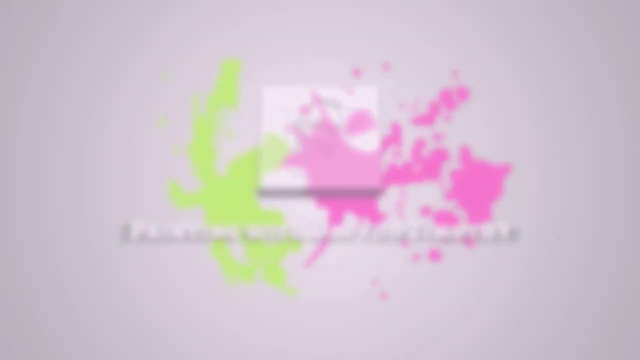 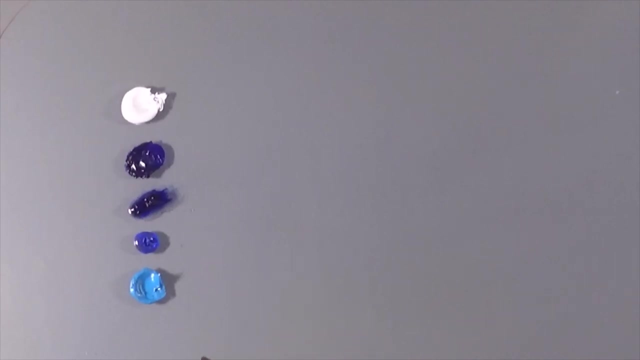 Today we're going to have a look at two different approaches to achieving realistic sky blues. Okay, one of my favourite subjects this- Skies and trees- were pretty much all I wanted to paint when I first started out, but, yeah, they held a special place in my heart. I'm going to show you. 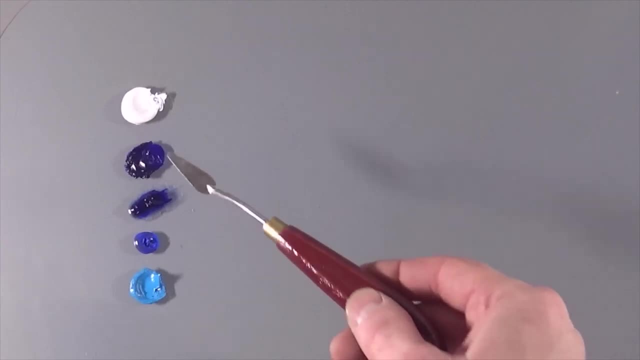 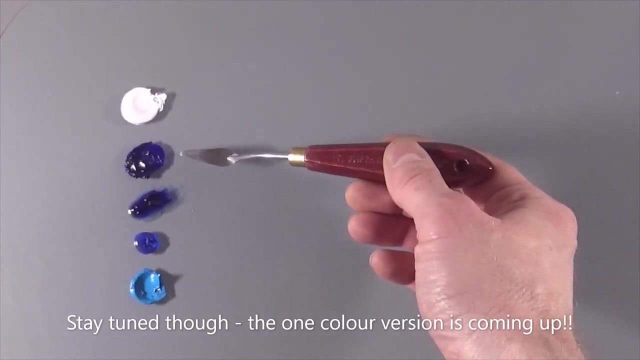 the colour gradient here in the form of four piles of paint as opposed to just the one that you really need to do this exercise, And that is basically from top to bottom. the sky starts off with a kind of a violet ultramarine. violet tinted into the blue works really nicely, We can use.